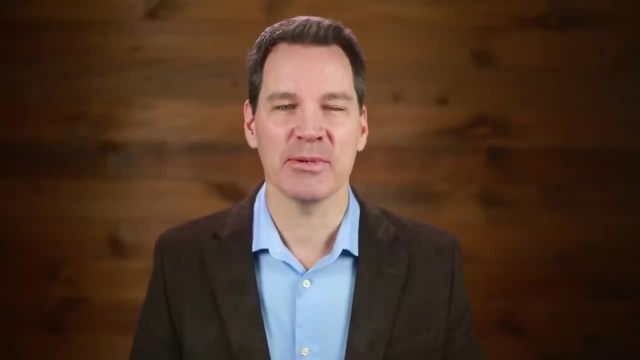 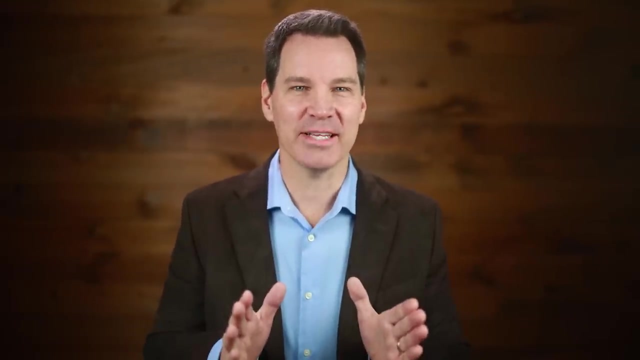 a concise story. A story is a high risk way to open, but it also has the highest potential rewards. So let's maximize those rewards and minimize the risks. One way to contain the risks is to make sure your story relates directly to the rest of your presentation. 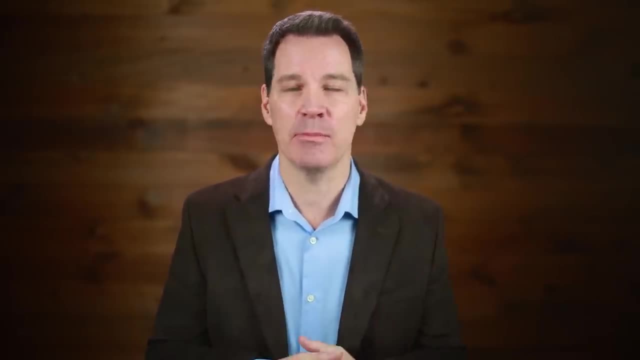 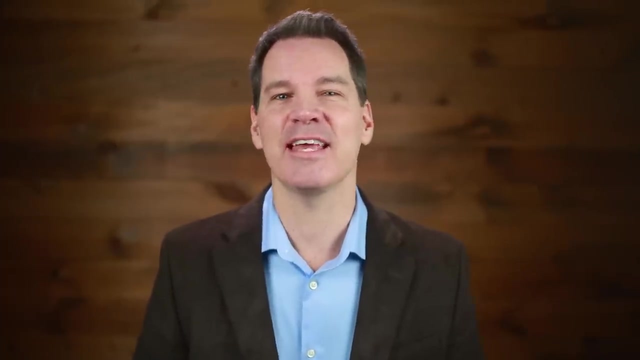 Now it could be a great story, but if it doesn't relate to the heart of your message, then people will wonder why you told the story. So find a story that fits the rest of your message. Another risk is telling a long winded story. 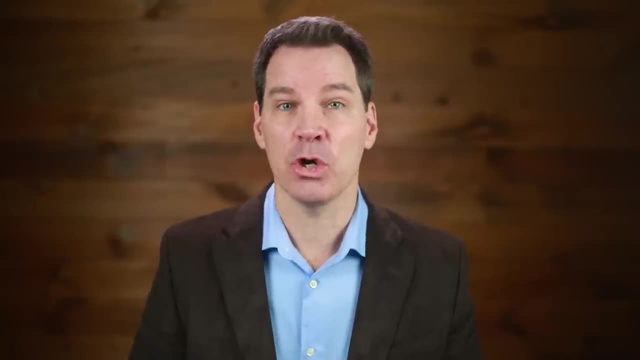 Make sure you're concise. aim for 30 seconds or maybe a minute for an opening story. Inexperienced storytellers tend to go on and on and weave all over the place. If you open with a long winded story, it will kill the energy in the room. 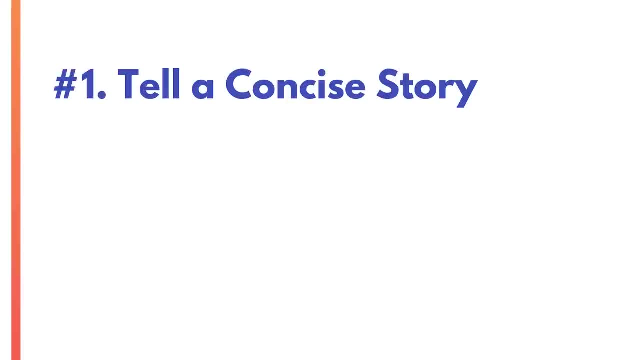 Practice until your story is concise. A good story also has a clear structure or logic. Story should have a beginning, middle and end, and then a lesson learned. The beginning can be one sentence and explain the people, time and place. 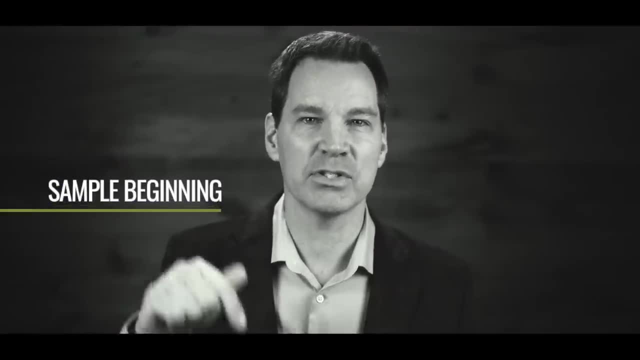 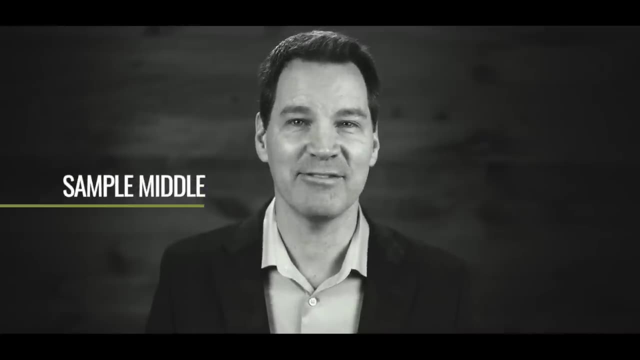 About six years ago, I started a YouTube channel right here in this room. The middle of the story is where the action takes place. I had a goal, but what I didn't have was any experience making videos. Up till then, I didn't even own a camera. 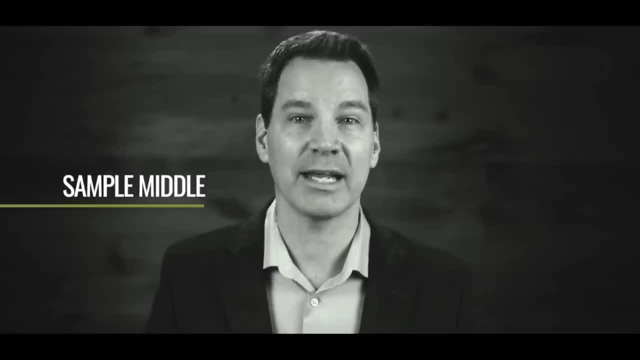 I knew nothing, but I started making videos every week and I learned as I went along, And six years later I've posted over 200 videos and the channel now has over 400,000 subscribers. The middle of the story is usually where people overcome some struggle. 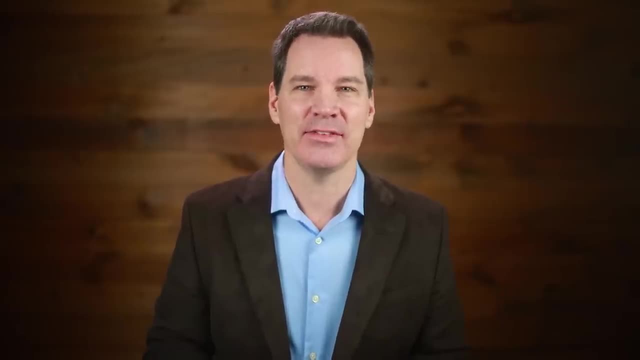 The endings to stories are usually pretty concise as well. The success of the channel has truly changed my entire life and led to opportunities I would have never been able to enjoy otherwise. The last part is called the lesson learned. You could also call this the moral to the story. 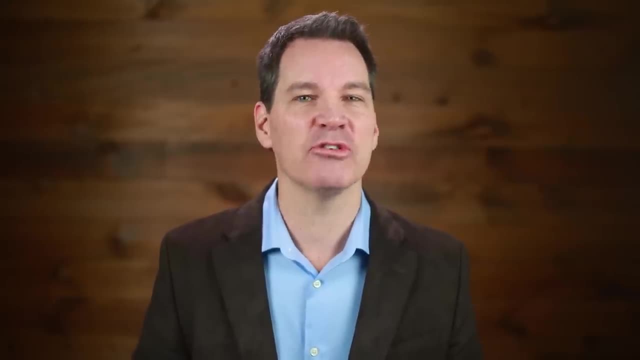 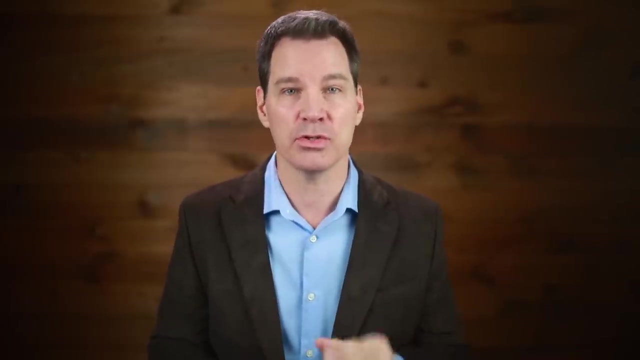 This is the key insight you want your listeners to remember. This long journey taught me what John Maxwell always says: everything worthwhile in life is up hill. If we put that whole story together, we'd last about 30 seconds or so. That simple structure will also keep you on track. 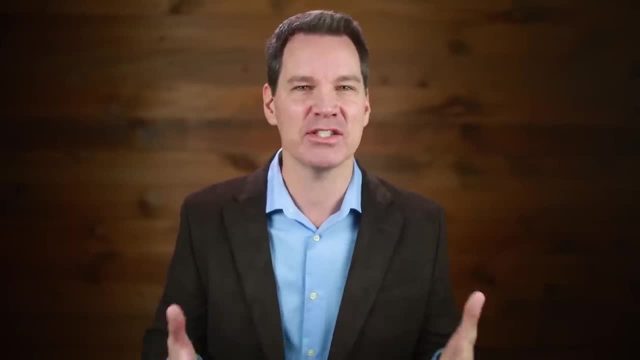 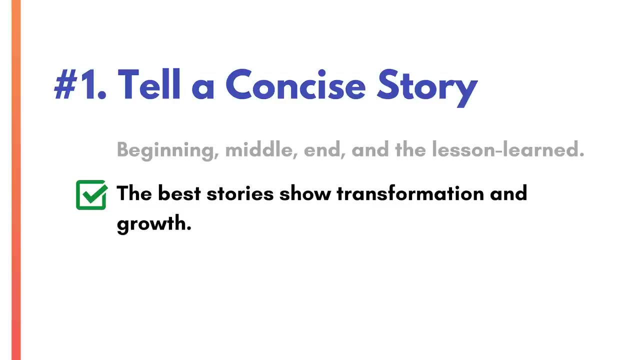 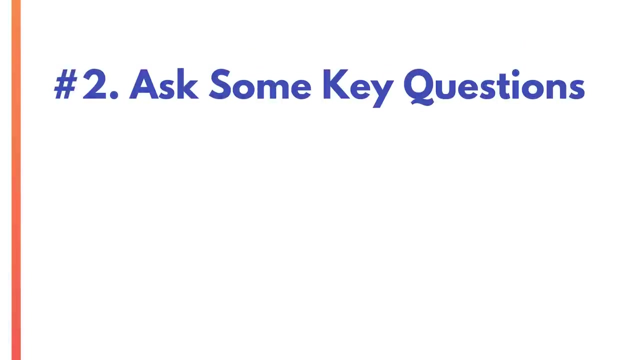 so you land on the right spot at the end then can give the rest of your speech introduction. The best stories show some transformation or growth. That's why stories have the highest potential reward as an opening. People love stories that have that before and after quality. 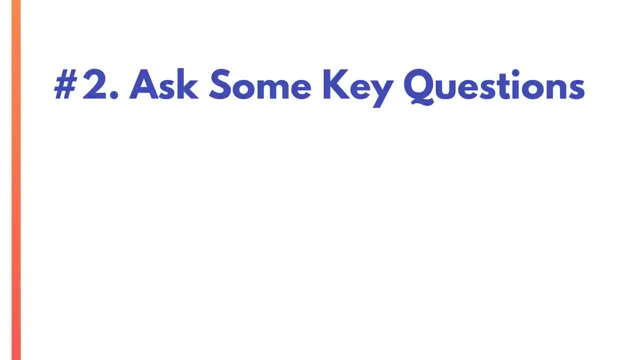 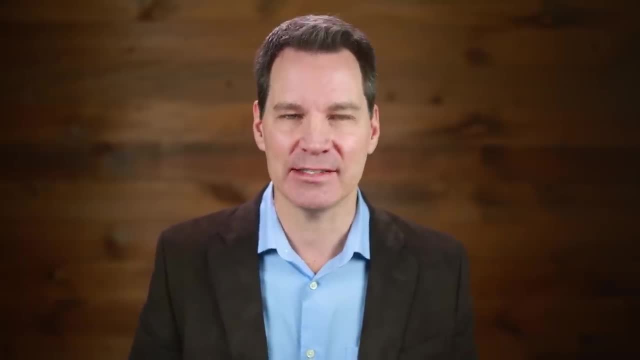 The second way to open a speech is by asking your audience some key questions. This is a really common way to start a speech. Some people say it's overdone, but I'll give you some tips to enhance this a bit On the plus side. 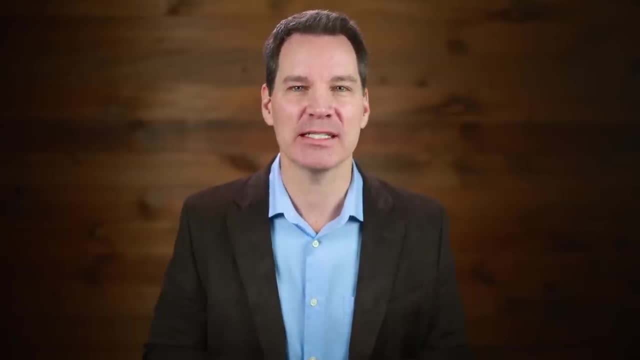 asking relevant questions can create instant engagement because it helps listeners see themselves in your presentation. I don't recommend you ask listeners to answer your questions out loud right at the beginning. That could take your presentation in the wrong direction. but ask questions that engage our minds. 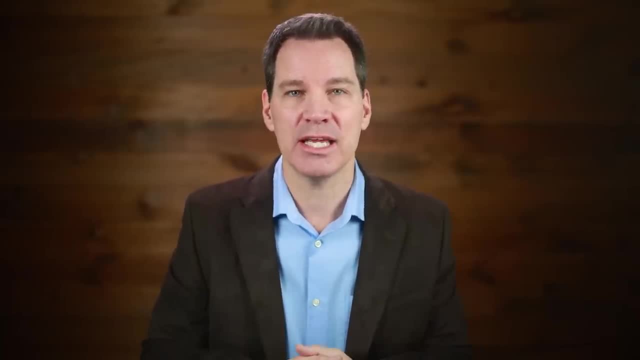 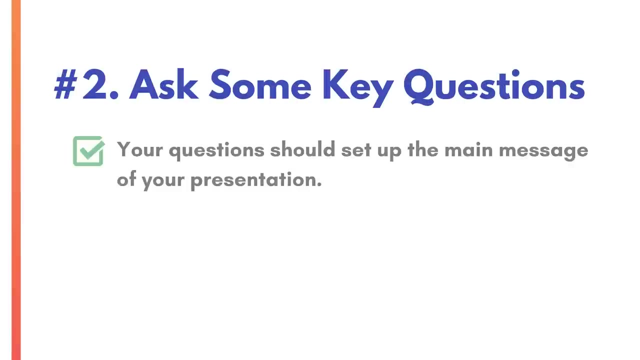 because that will draw us into the world of your presentation. in a mental conversation. Questions peak our curiosity. Now here's some tips to enhance your questions. First, make sure your questions set up the main message of your presentation. You want to ask questions that your speech will respond to. 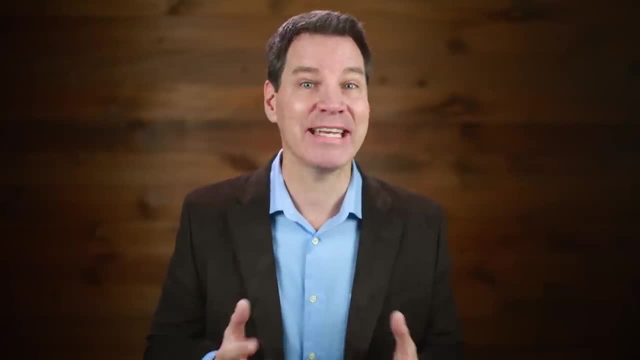 in some satisfying way. So let's say I was doing a presentation on financial planning for retirement, I might ask if you could retire to a dream location. where would that be? That question can easily lead right to my main message about retirement planning. 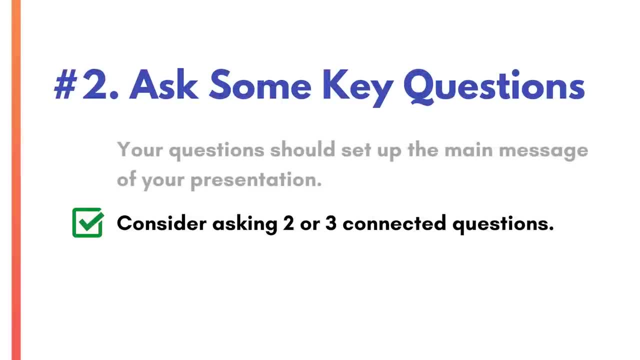 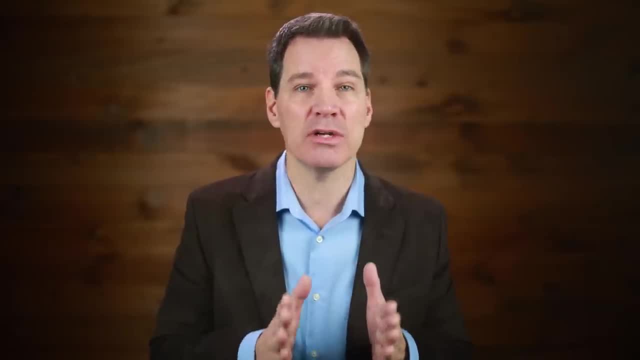 Second, enhance it more by asking two or three connected questions rather than a single question. Questions usually go by a little too quickly, So ask two or three and pause briefly in between. That will build momentum. So I'll go back and redo the first sample question. 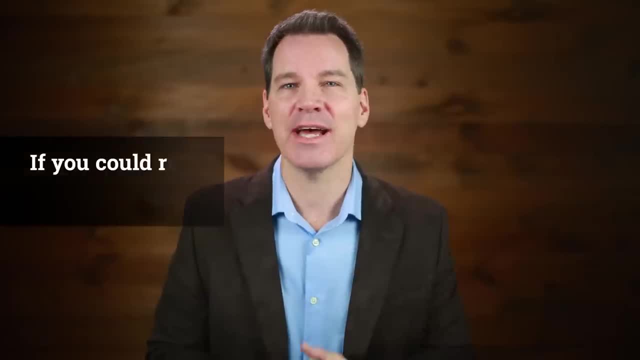 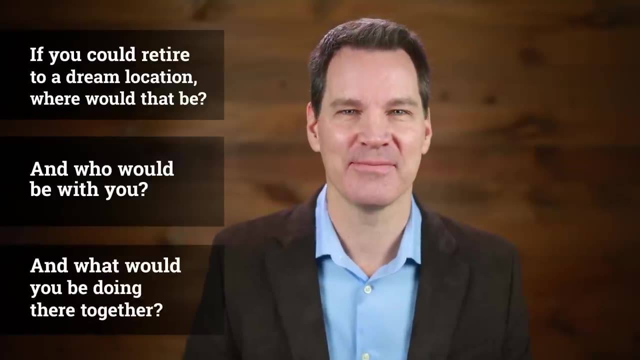 and add two more questions with pauses. If you could retire to a dream location, where would that be And who would be with you And what would you be doing there? together Each question is really concise, but when you add them together, 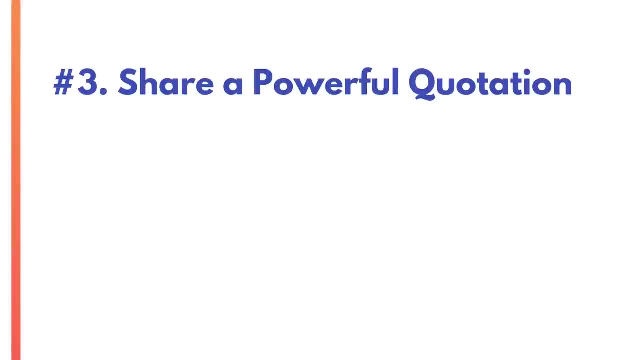 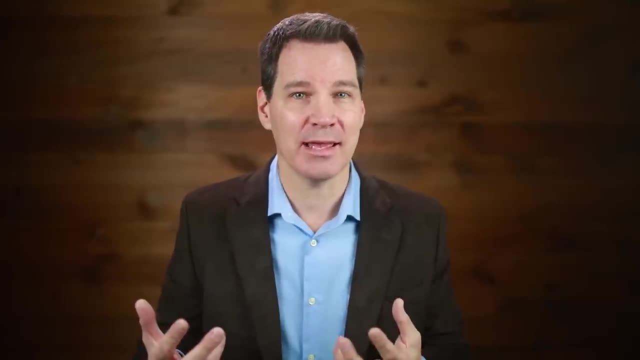 they create more engagement. Third, open by sharing a powerful quotation. Quotations are great openings because we can always find somebody who said what we're trying to say with even more impact, And the great thing about quotations is that they've already stood the test of time. 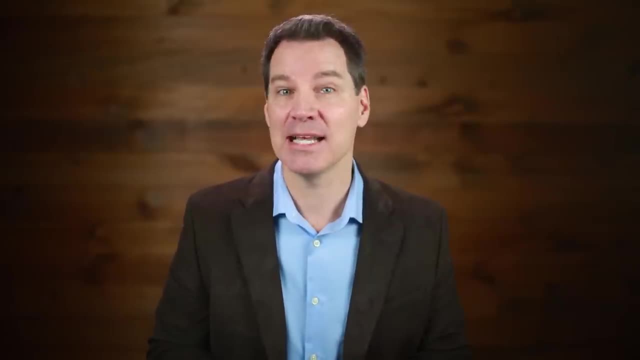 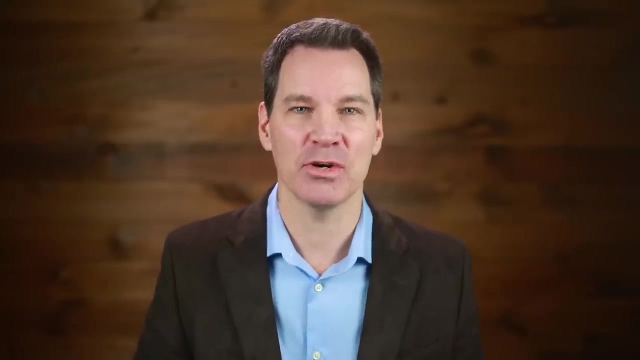 If it's the kind of passage that people quote, then it will likely have a positive impact on your listeners as well. So let's say I was doing a speech about the importance of creating a big, ambitious vision for our lives and chasing our dreams. 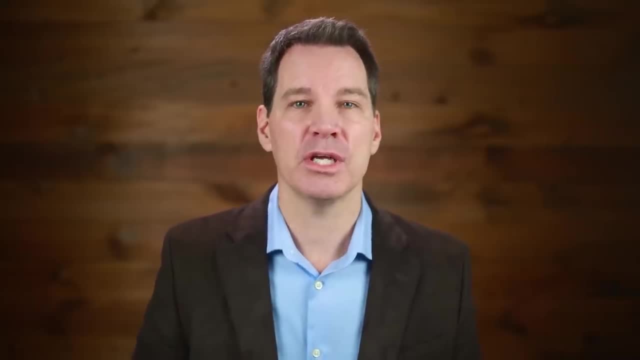 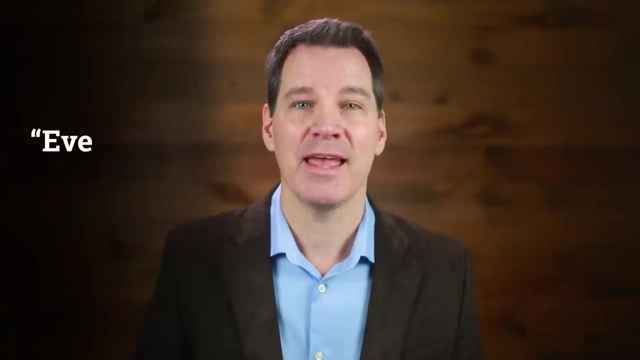 a topic that I am very fond of, by the way. I might open with a quotation like this, a quotation I mentioned a moment ago: The famous writer John Maxwell, who wrote the famous book. John Maxwell has often said: everything worthwhile in life is uphill. 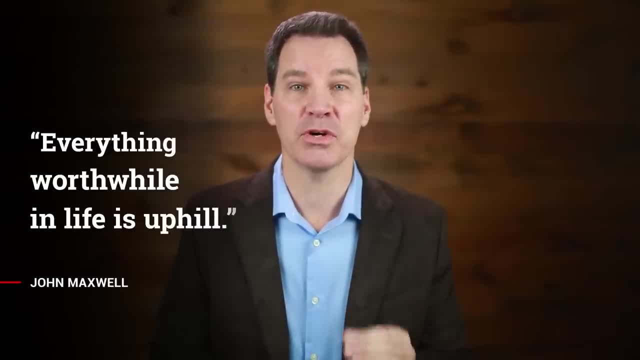 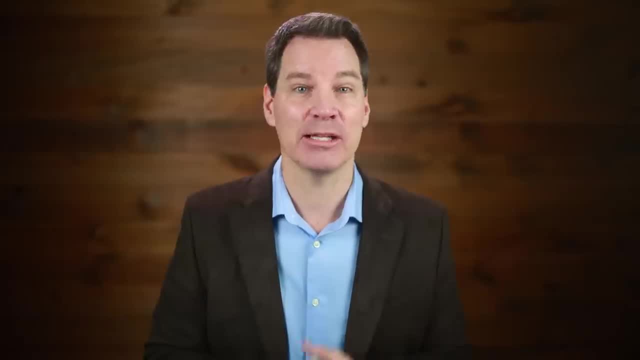 A couple of tips on using quotations. Make sure the person you are quoting actually said or wrote those words. I saw this quotation come out of John Maxwell's mouth myself and I looked up later to double check it. You don't want to get a quote wrong. 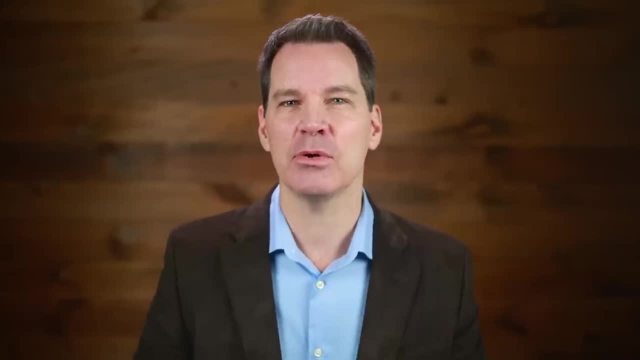 or attribute it to the wrong person. The key, though, is to find a quotation that makes an impact and relates directly to the heart of your message. Just like all the other ways to open a speech, the quotation should be a natural jumping off place. 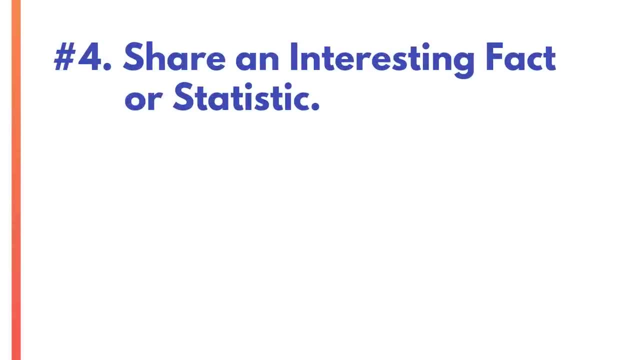 for whatever comes next in your introduction. Fourth, open with an interesting fact or statistic. This works really well if you have any concrete data. that's a little bit surprising. As you're preparing, you might come across a bit of information and you say to yourself: whoa, I didn't know that. 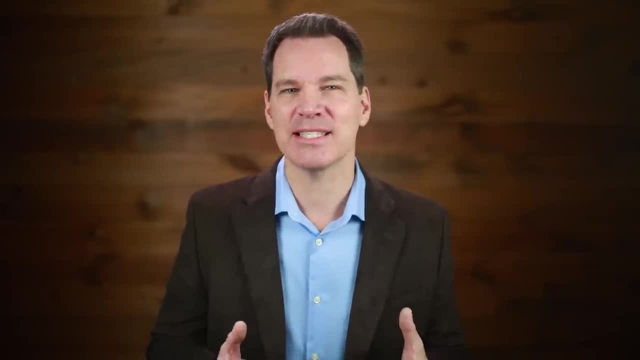 If a statistic or fact grabs your attention like that, it will likely have a similar impact on your listeners. For example, the other day I was looking up information about getting struck by lightning, because people around me- people around me- are getting struck by lightning. 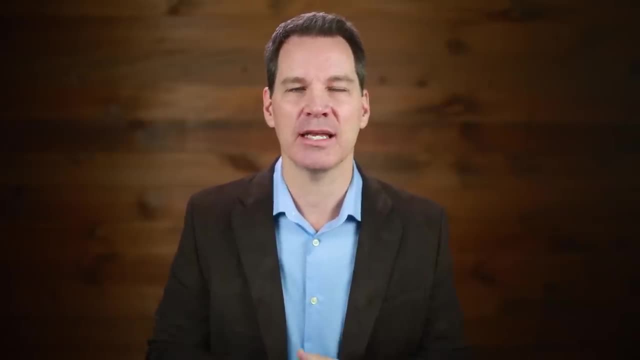 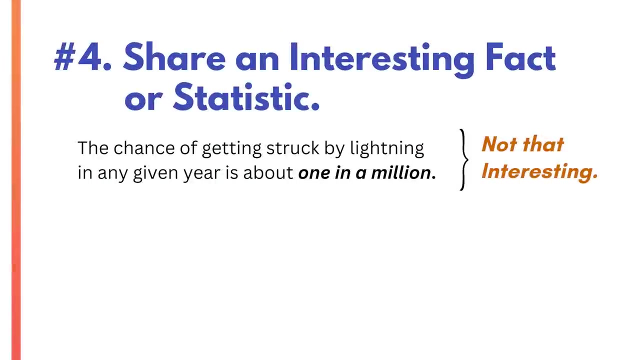 Because people are always using the chances of getting struck by lightning as a point of comparison And the first statistic I found wasn't all that interesting. The chances of getting struck by lightning in any given year is about one in a million, So struck by lightning equals one in a million. makes sense. 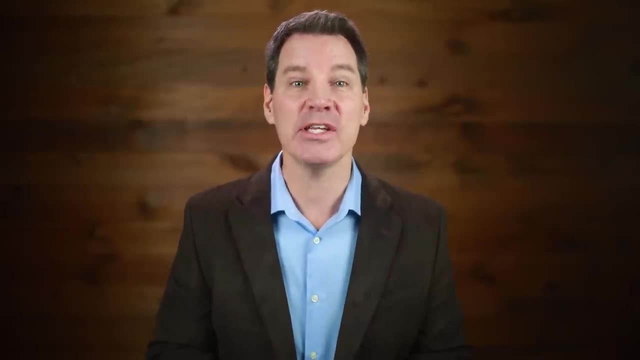 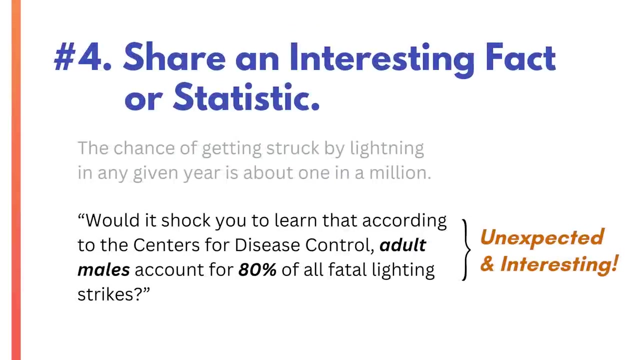 But then I noticed another statistic that did surprise me, And here's how I might share that in a speech opening. Would it shock you to learn that, according to the Centers for Disease Control, adult males account for 80% of all fatal lightning strikes? 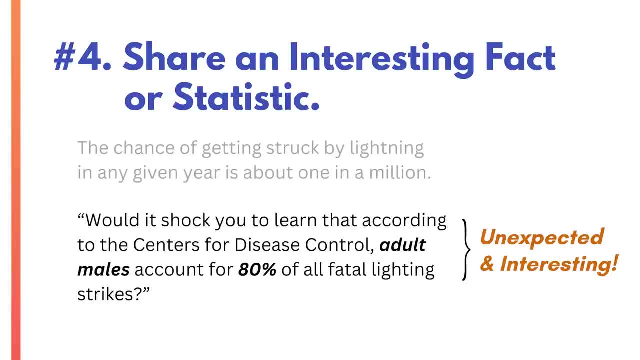 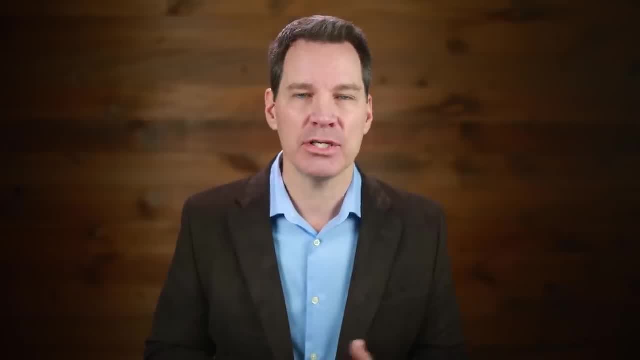 To me that was an unexpected statistic And I wanted to learn more. I told that to a couple of friends and they both said: really, The takeaway for you is that as you're doing your preparation research, you may find yourself surprised or wanting to know more about what you're reading. 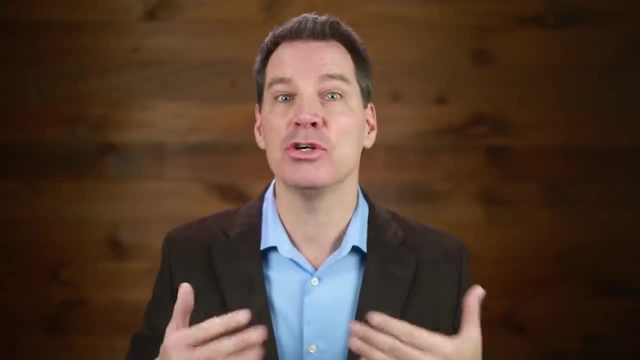 That's when you know you've come across a fact or a statistic that could be a very good hook That will make the audience want to pay attention to the rest of your message. The trouble with facts and statistics as an opening is that it's not just facts and statistics.